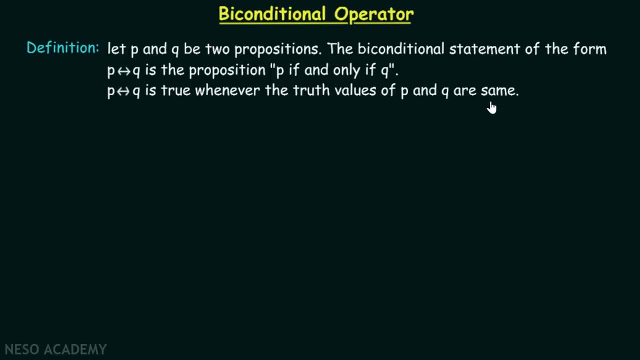 of P and Q are same. Let's consider the truth table in order to understand this point in a better way. Now, when truth values of P and Q are same, then only we would be able to get the compound preposition true, As you can see from this truth table. 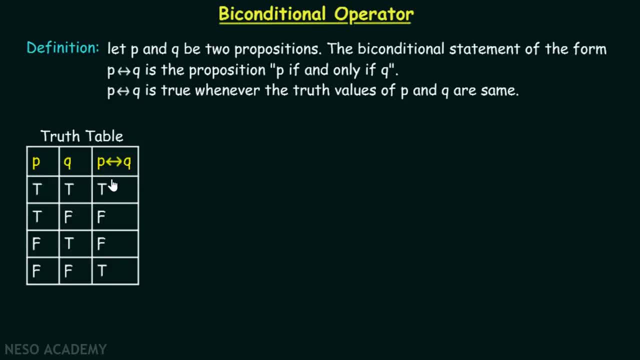 That is, when P is true, Q is true, then we will get the compound preposition true. And when P is false, Q is false, then also we will get the compound preposition true. Otherwise, the compound preposition is simply false. 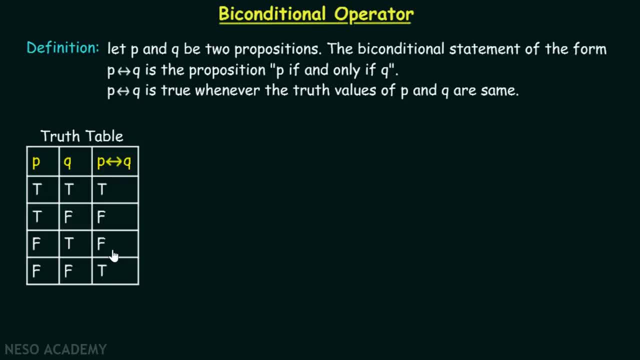 Now why it is the case. Biconditional simply means not only P is sufficient for Q, but P is necessary for Q as well. Therefore, we can say that when P is true, then Q has to be true, And when P is false. 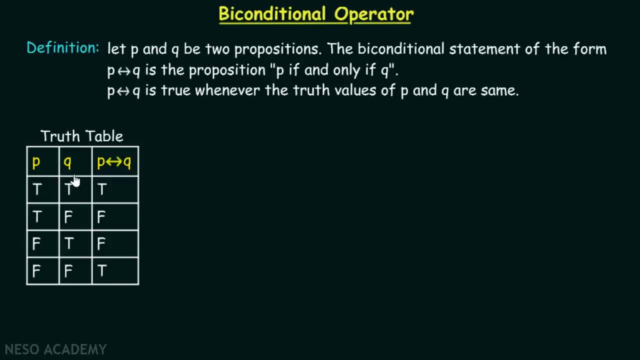 then Q has to be false. Similarly, we can also say that when Q is true, then P has to be true, And when Q is false, then P has to be false. That is the reason why only for these two combinations we have the compound preposition true. 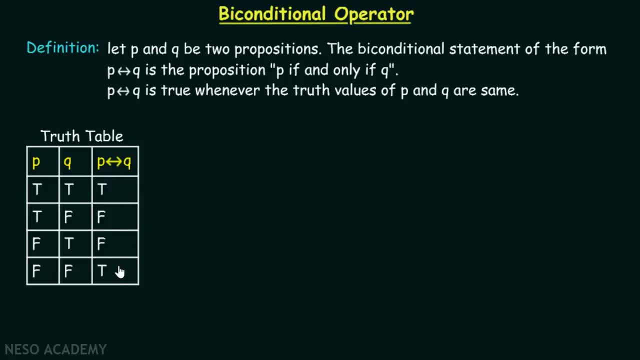 Okay, Now let's consider one question: How P, if and only if- Q makes sense. Now let's try to understand why. why we are writing if and only if, in between P and Q, to indicate the biconditional statement. Let's try to understand this particular point. 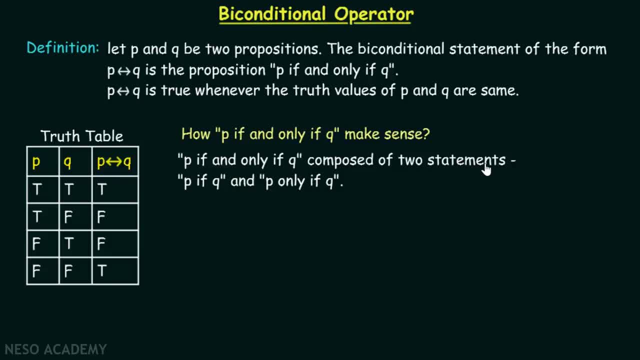 P if, and only if, Q is composed of two statements: P if Q and P only if Q, Isn't that so? It is the combination of these two statements: P if Q and P only if Q. Now let's try to understand them separately. 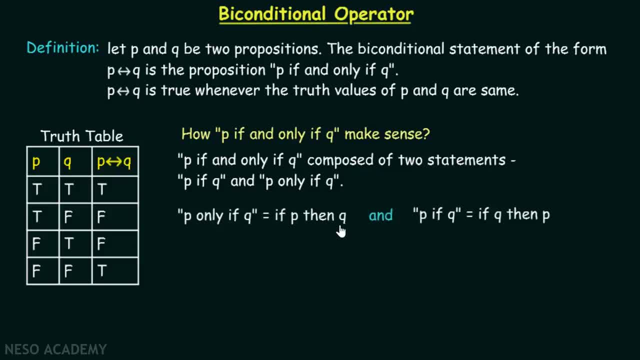 P only if Q simply means if P, then Q and P. if Q is equivalent to if Q, then P, Isn't that so Now, as because a biconditional statement is the combination of if P then Q and if Q then P, 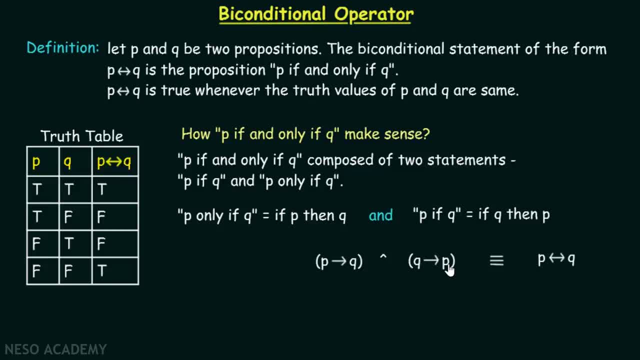 it looks like P implies Q and Q implies P. We can combine them together to represent this particular compound preposition, That is, P biconditional operator Q. This biconditional operator comes from these two implication operators, That is, forward arrow from P to Q. 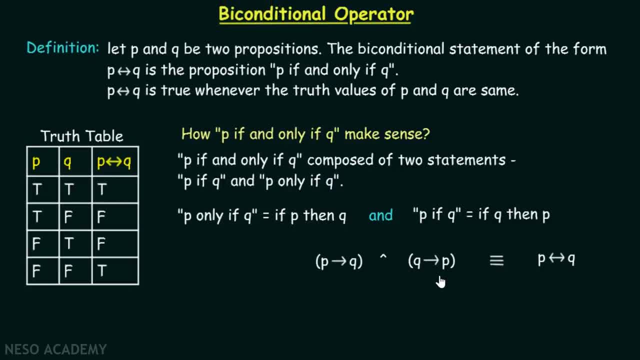 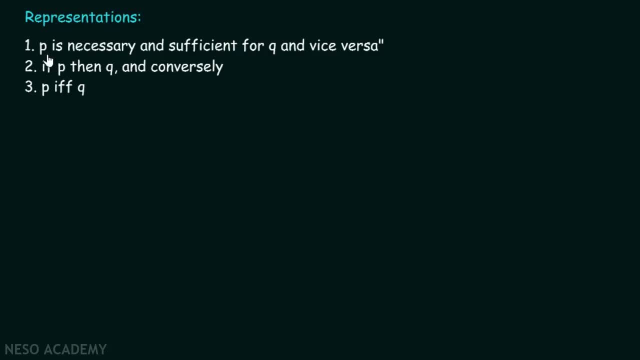 and backward arrow from Q to P. Now let's consider the different ways to represent the biconditional statement. Not only we can say that P if, and only if, Q, but we can also say that P is necessary and sufficient for Q. 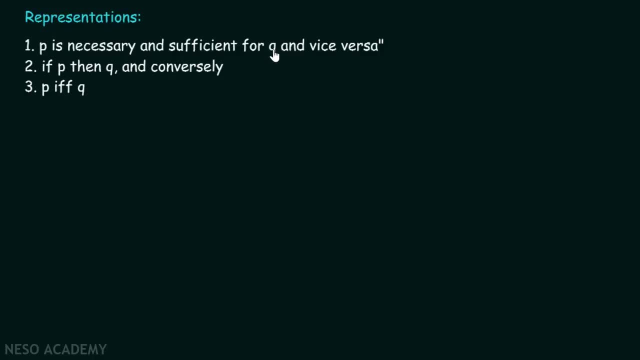 And we can also say that Q is necessary and sufficient for P Right. If P, then Q, and conversely is also one of the representation of biconditional statement. P if and only if Q can also be written in short form as P if Q. 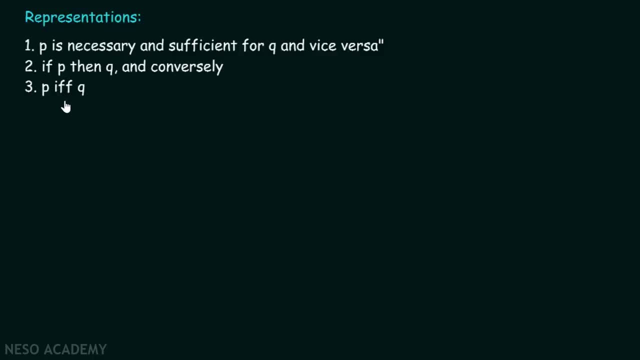 Please note down: it is not I f. if It is I f f. if It represents if and only if. Let's consider one example in order to understand how we can write biconditional statements if we have two prepositions: P and Q. 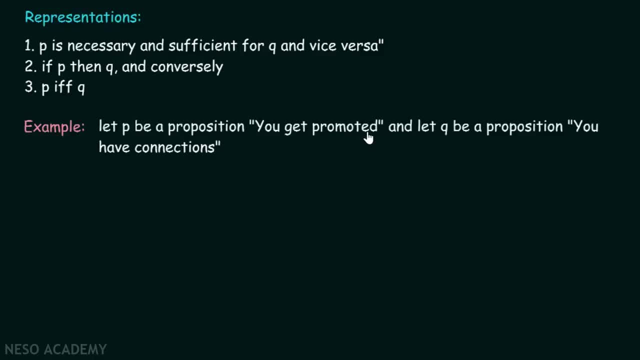 Let P be a preposition: you get promoted and let Q be a preposition: you have connections. Then P if and only if. Q is the statement. you get promoted if and only if you have connections. As simple as that. Now, this particular compound preposition is true. 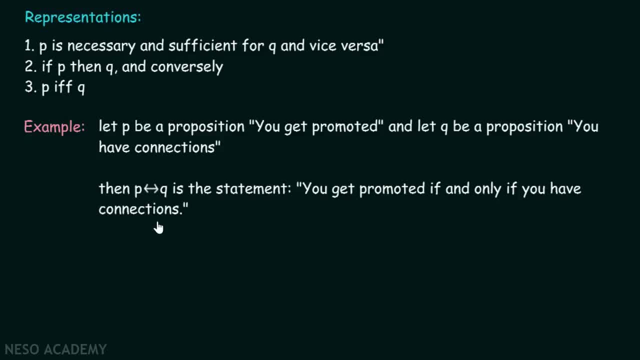 whenever P is true and Q is true, or whenever P is false and Q is false. You get promoted if it is true and you have connections. if it is true, then definitely this compound preposition is true If you haven't get promoted and if you have no connections. 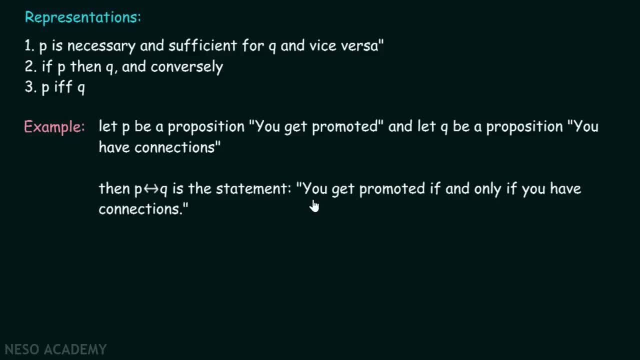 then also this compound preposition is true Here: if you get promoted but you have no connections, then this compound preposition is false, Because, according to this statement, you get promoted if, and only if, you have connections. Now you get promoted and you have no connections.